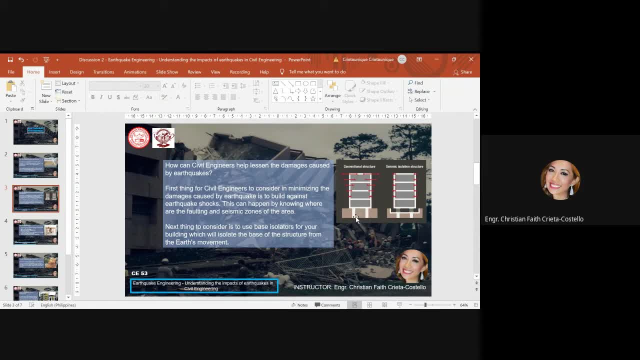 wherein the foundation is just erected straight directly into the ground. However, for a structure with seismic isolation, you can see here the base isolators. there are many kinds of base isolators: It could be a spring or it could be rollers made of huge steel ball. 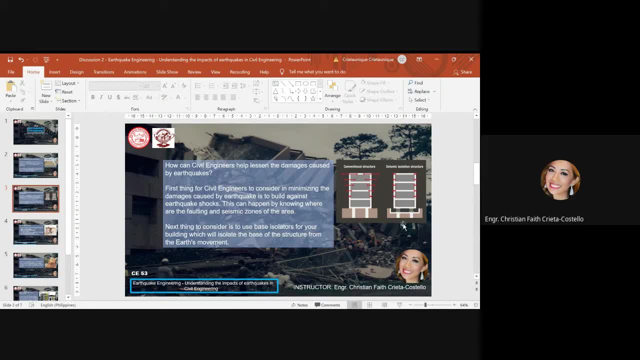 Later in our discussions we will also dig deeper into how seismic isolation will be done. Also, some structures, especially if these are tall buildings, they are using pendulums to balance the weight if shaking will happen. And another thing is the main reason of high-rise buildings like condominiums and hotels. 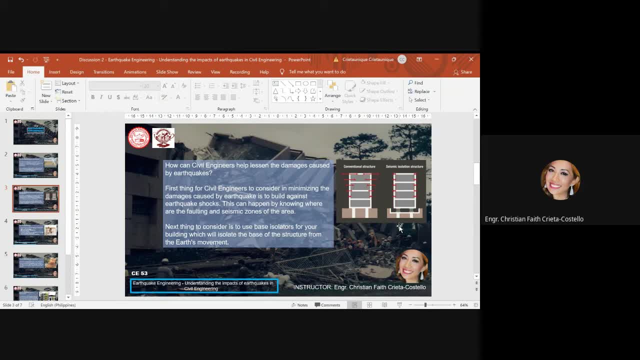 why they are putting swimming pools on top of the building is because the water and the swimming pool itself will counteract the movement during the shaking of the earthquake, So it will have the same purpose as a seismic isolator or the base isolator. 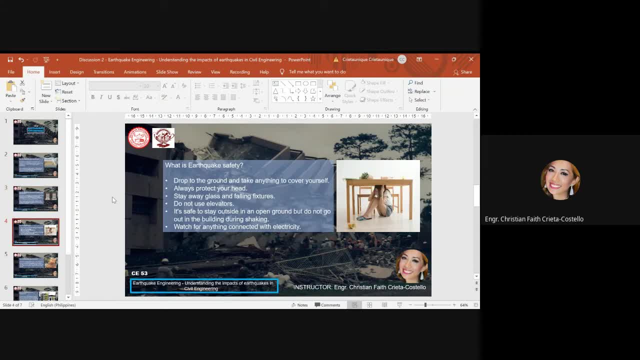 Next is: what is earthquake safety? This is applicable to anybody, not only for civil engineers. First, is you need to drop to the ground and take anything to cover yourself. Then always protect your head. Stay away from, stay away from. 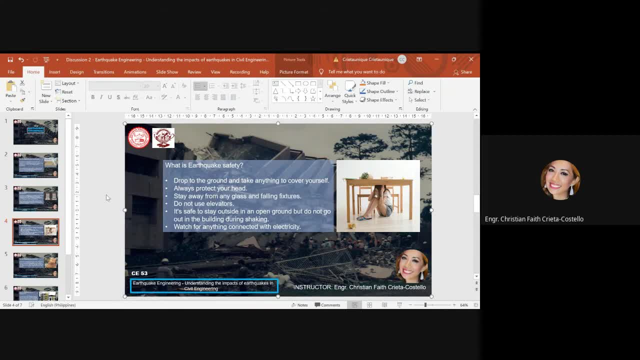 rainy glass and falling pictures. Do not use elevators. if you are in a high-rise building, Then it's safe to stay outside in an open ground, but do not attempt to go out in the building during shaking. Then watch for anything connected with electricity. 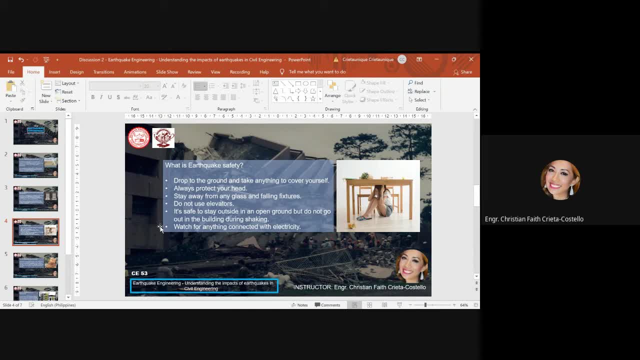 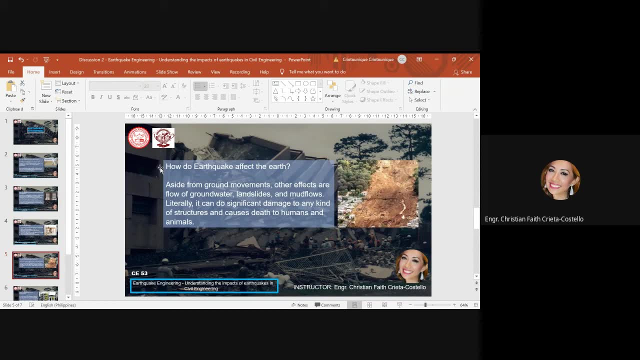 because anything can happen related to electricity during earthquake. Next is: how do earthquakes affect the earth? Aside from ground movements or the shaking, other effects that we can expect that earthquake can do towards our planet is the flow of groundwater or the increase of flow. 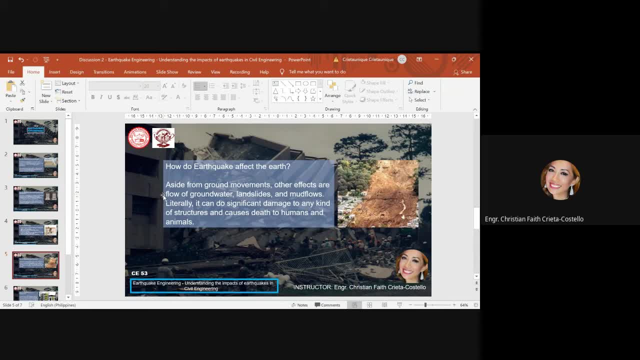 there could be floods that will happen, then landslides and then mud flows, So literally it can do significant damage to any kind of structures and can even cause death to humans and animals. That's what you can see here in the photo. 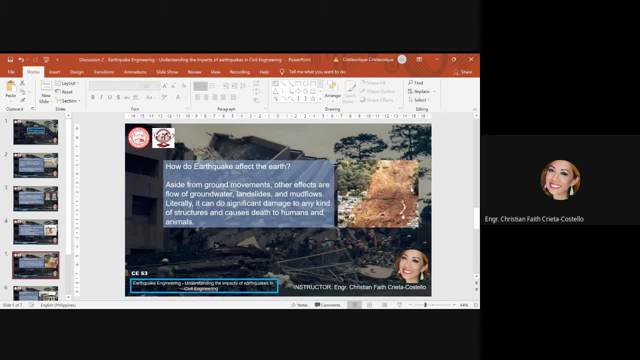 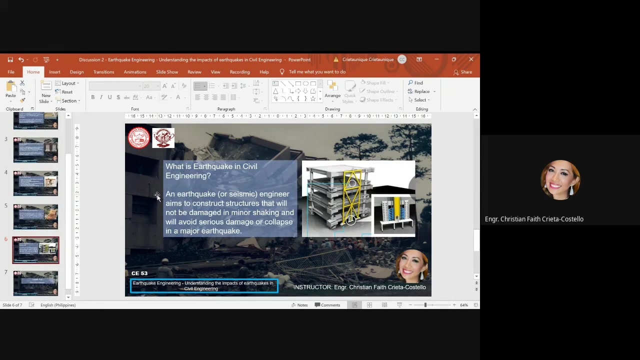 There's a landslide happening from the mountainside and then totally covering the households, that is directly affected of the catastrophe, Then what is earthquake in civil engineering? So an earthquake or seismic engineer always aims to construct structures that will not be damaged in minor shaking. 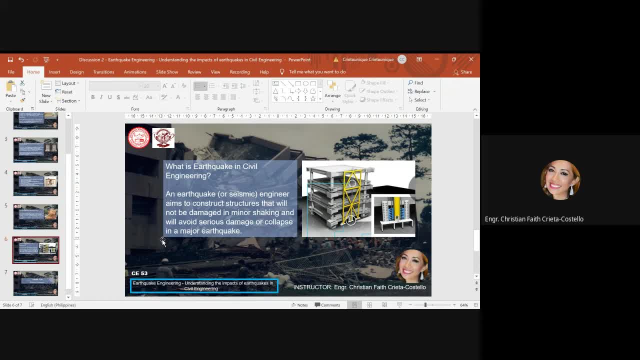 and will avoid serious damage or collapse in a major earthquake. Literally speaking, we cannot really prevent earthquake to happen, but at least as a civil engineer with the knowledge of earthquake design- especially if you will study further into being an earthquake engineer or seismic engineer- 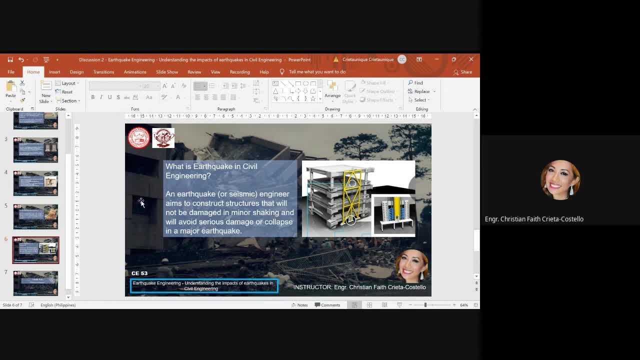 then you can really do a bigger job in avoiding or not avoiding, in minimizing the after effect or the serious damages that could happen to the structure, to avoid these major accidents and then major situations that can really even cause death to people. And then 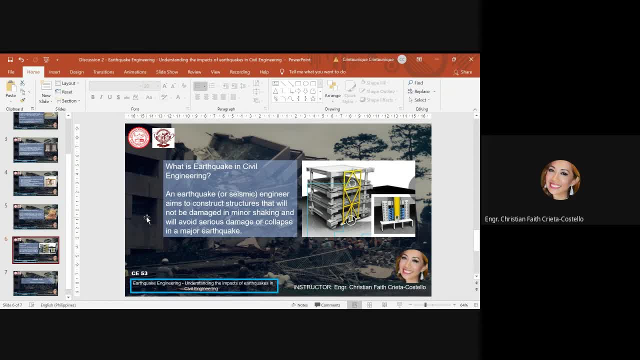 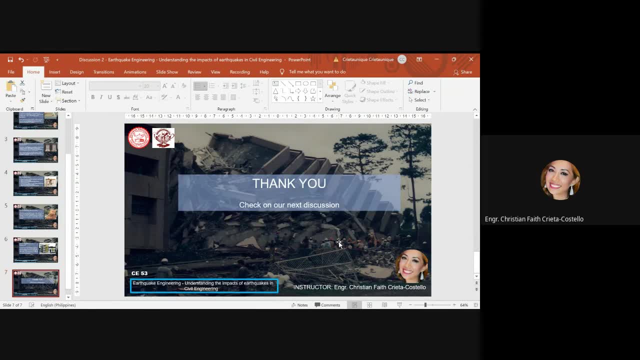 of course, to avoid the total collapse of a structure that you are designing. So that is all. You can check further in our next discussion.